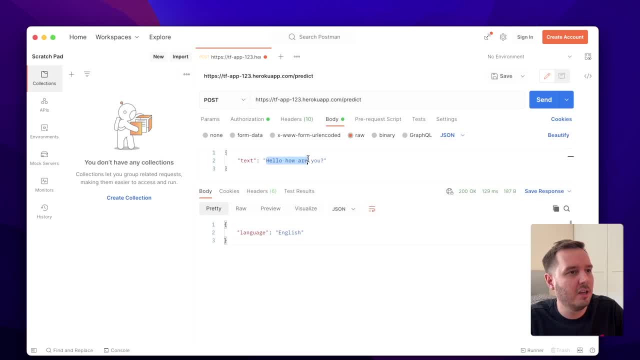 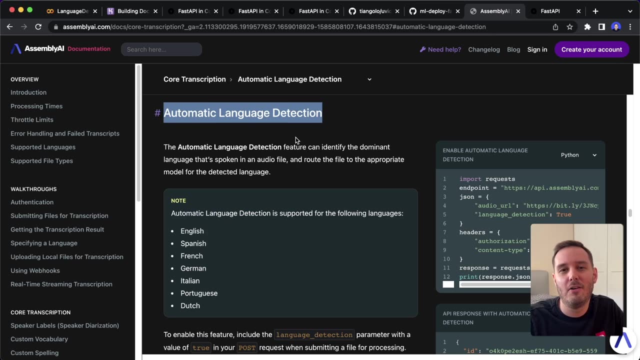 on Send, we get this response with languages English. If I, for example, switch this with the German version and click on Send, then the language should be German. So this is correct And fun fact on the side at assembly AI, we also have a automatic language detection feature in our API, So this is actually a 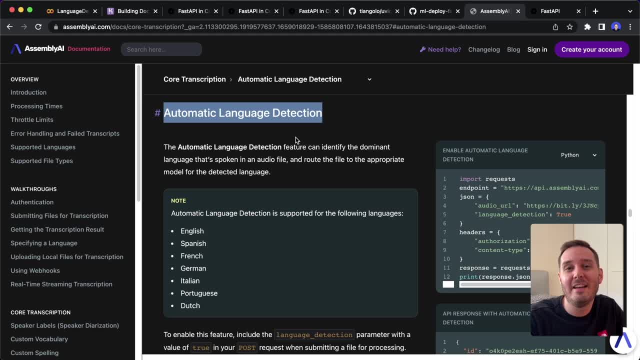 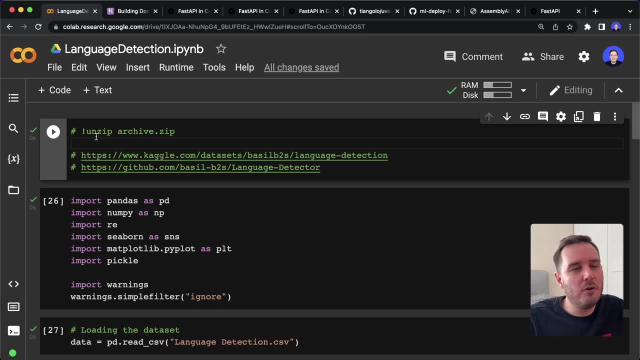 real world project. So let's see if we also can develop an accurate model and deploy this. So first let's build and train the model in a notebook. So here I'm in a Google Colab And the focus of the video is not how we develop this specific model, but rather how we go. 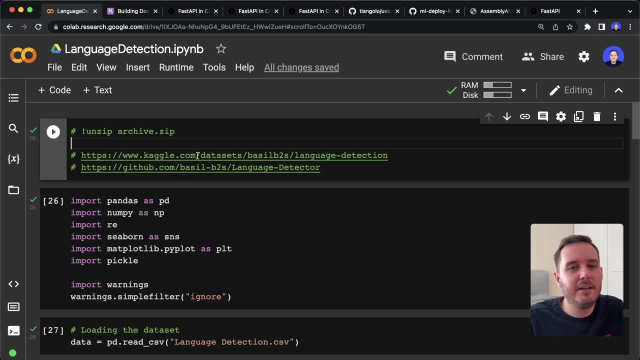 from notebook to production app in a moment. So let's go over this very quickly. The data set is available on Kaggle Also. this notebook and all the rest of the code is available on GitHub- Click in the description. So here we have our imports, then we load the data set and 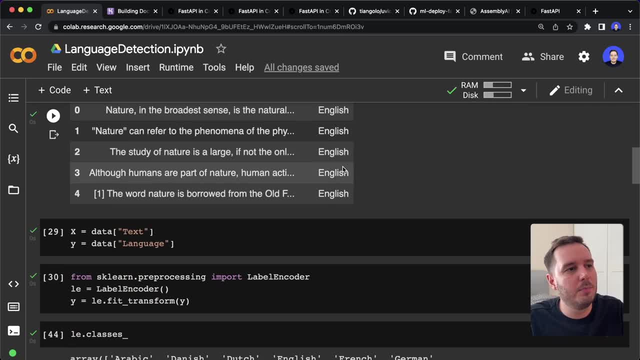 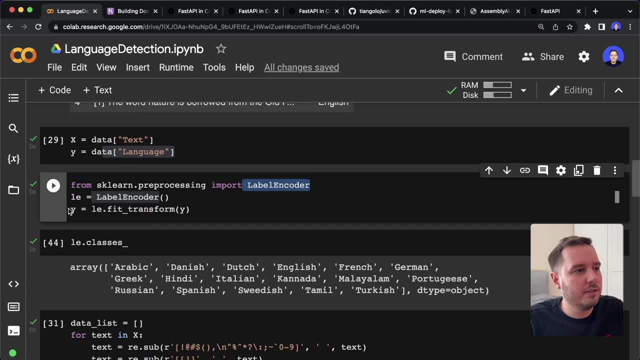 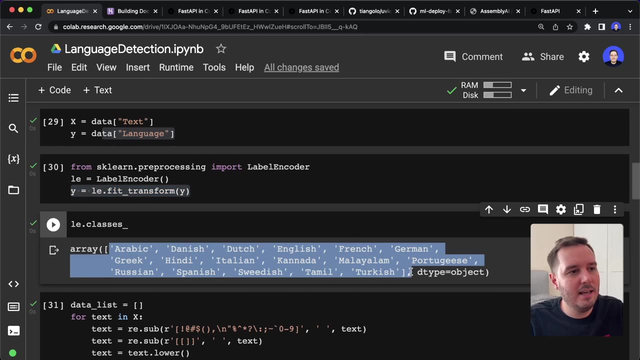 analyze this, So we have lots of different texts and the corresponding language. This is our x and y. then the first step we apply is a label encoder, So this transforms the labels y. So basically, what it does is that for each of these texts, these classes, it 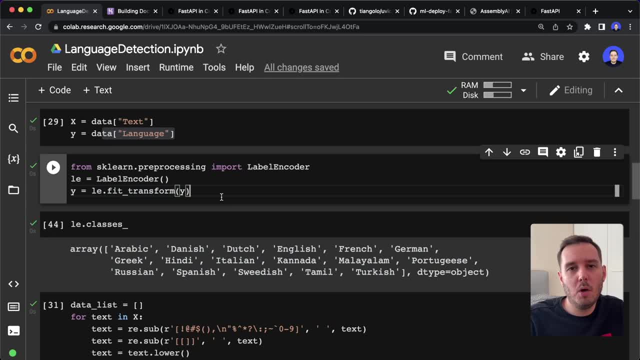 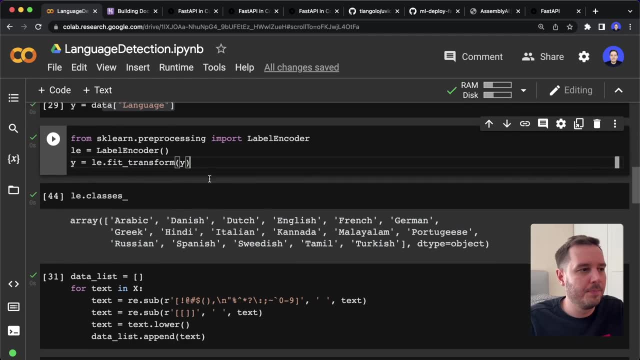 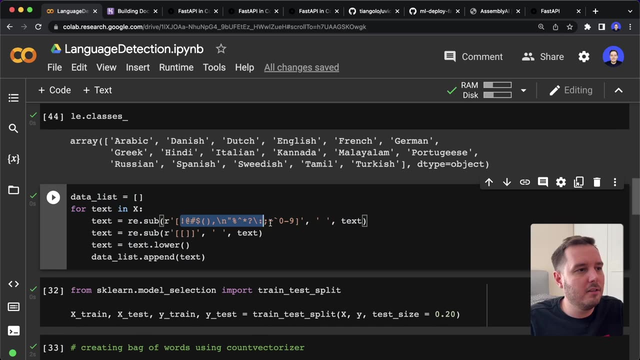 assigns a number starting from zero, And whenever we have a pre processing step that transforms our data, We have to remember this and later also use this in our code. So, for example, this is another pre processing step. Here we apply regular expressions to remove these special. 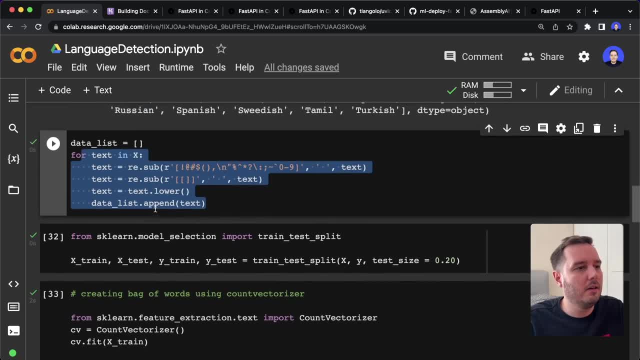 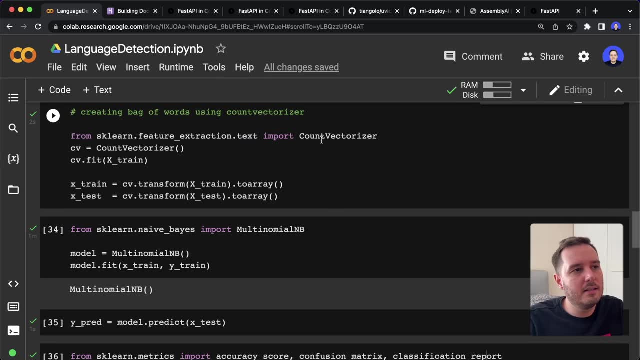 characters, So we also have to use this in the code later. Then we have the typical train test split And now we build our model. So it consists of two parts In this case. the first one is a count vectorizer. Here we fit this and then transform this, And then we 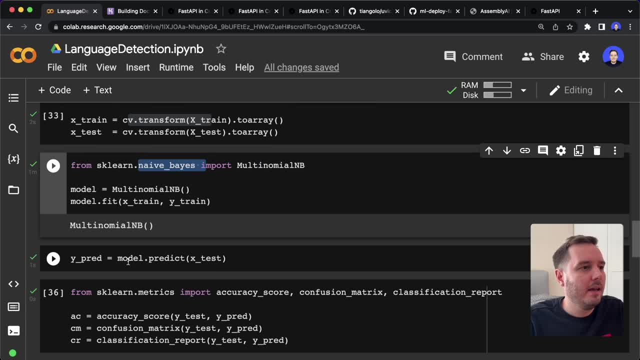 have the second step, which is a naive vectorizer. So here we have the second step, which is a naive vectorizer, And then we have the second step, which is a naive vectorizer, And then we have the second step, which is a naive bias model, And then we can use model predict. 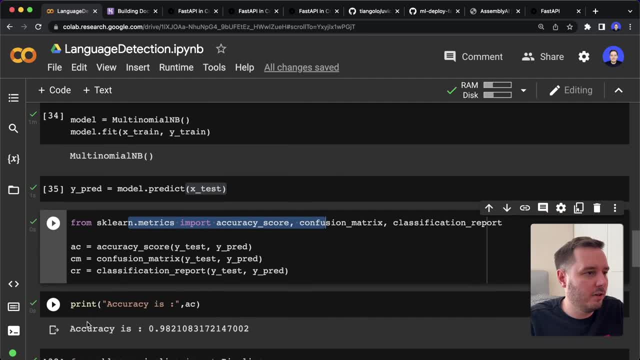 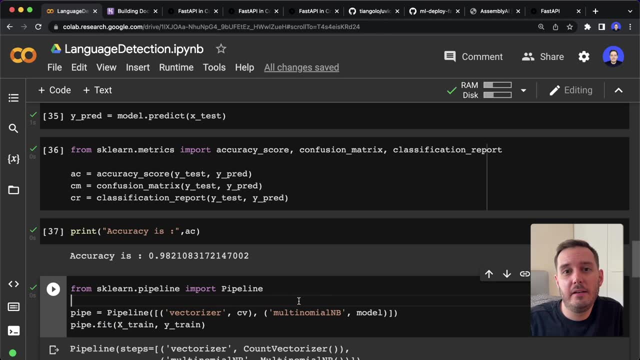 with the test data. And then here we have some metrics and, for example, print the accuracy, So we can see this is 98%, So pretty good. Now one best practice we can apply here, if it's possible, is to combine all steps into only one step. This is much less error prone. 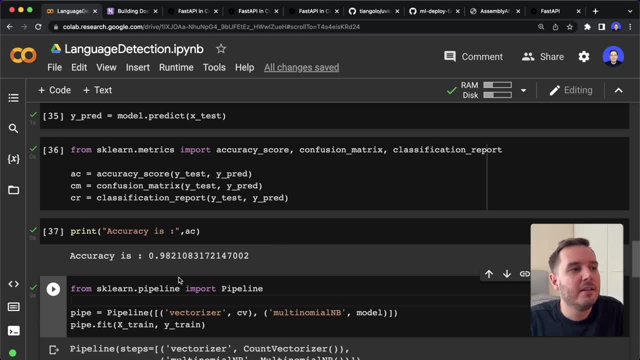 And then we only have to save one model instead of two here. So with sklearn we can do this with the pipeline. with TensorFlow, For example, we often have a sequential model where we can put in all the layers in this sequential model. So with the pipeline we can now combine. 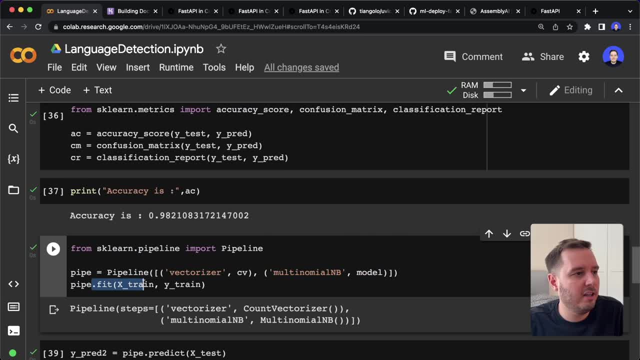 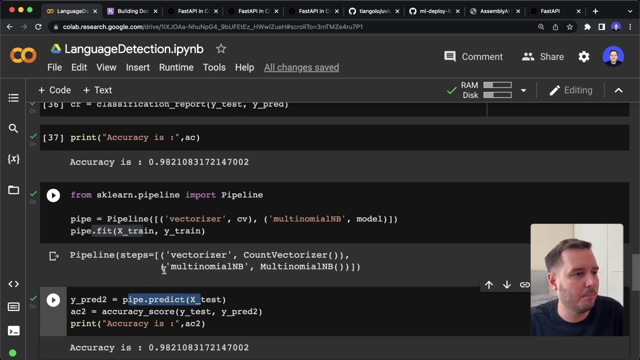 the vectorizer and the naive bias, and then we can fit the pipeline And then we can use this pipeline to predict the test set. So now we only have to apply this one step And if we compare the accuracy then we see this is the exact same result. So now, when we are 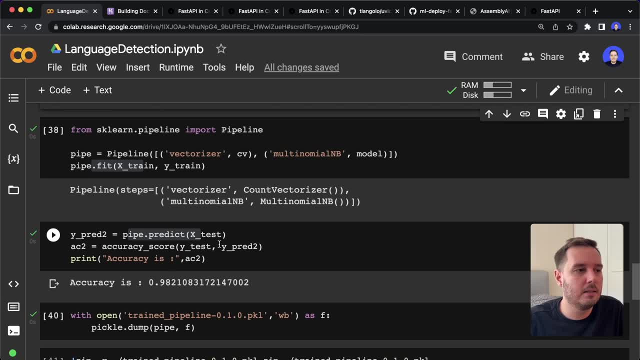 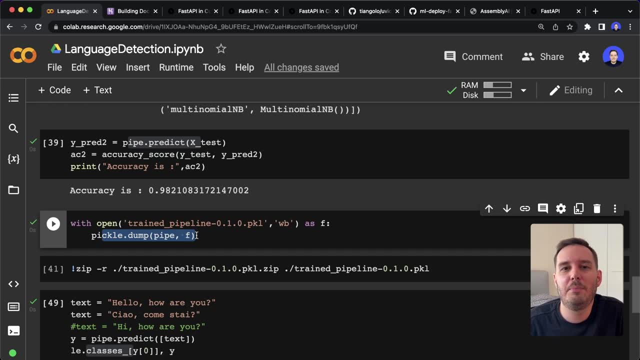 done with training the model. we have to save and download this, And with sklearn we can do this with pickle dump, So with TensorFlow and pytorch there's also a very simple API to save your model. One thing I recommend to do here is to also save a model version so you can keep track of the. 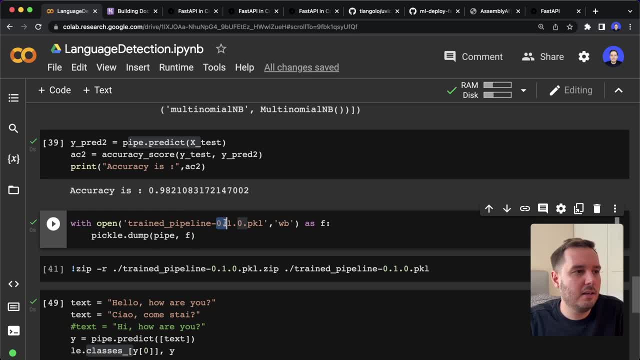 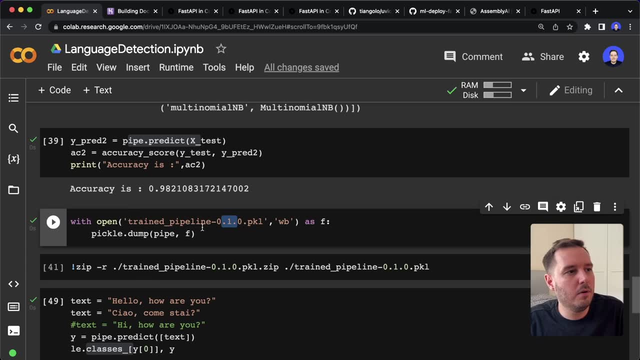 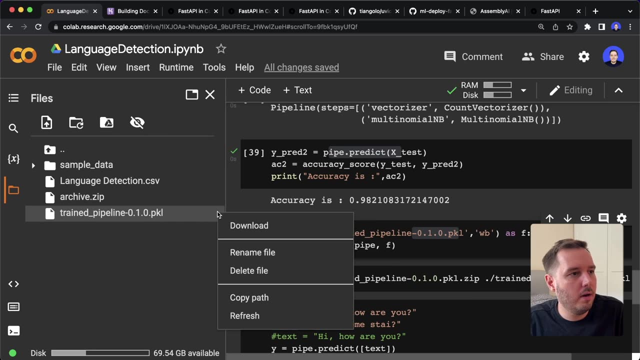 current version you have. So we use this syntax major, minor and patch version. So this is our first minor model version. And one other thing I want to mention here is that now, in this case, this will be one pickle file, So we can actually go ahead now and click on. 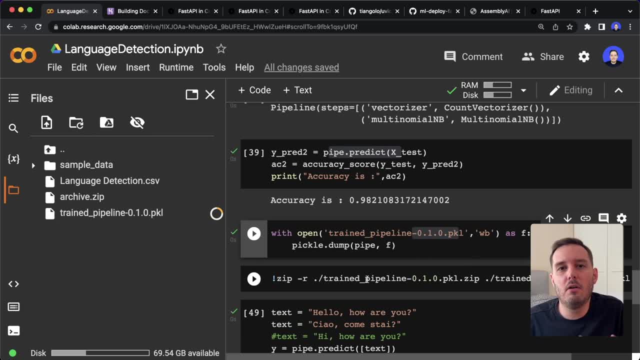 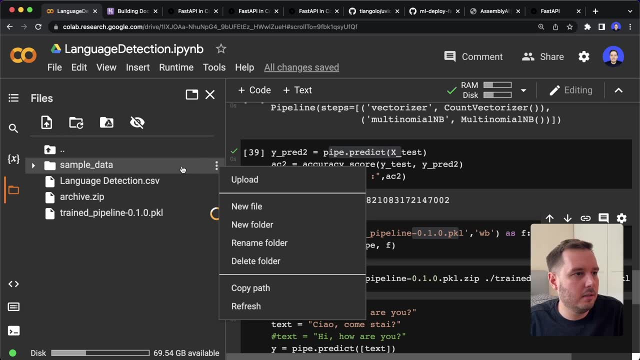 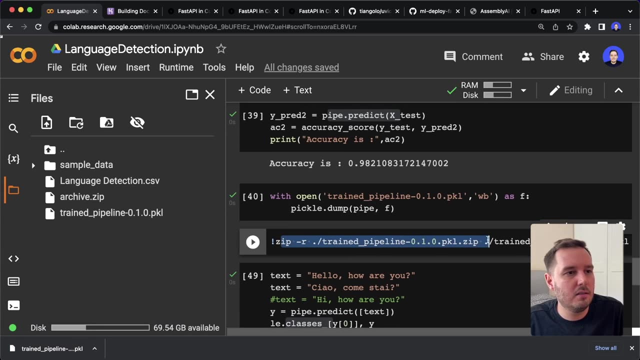 download here. But if you use TensorFlow or pytorch, then often it will save this in one whole directory And we cannot download a whole directory. So there's no download button. So one trick you can apply is to sip a folder with this command. So exclamation. 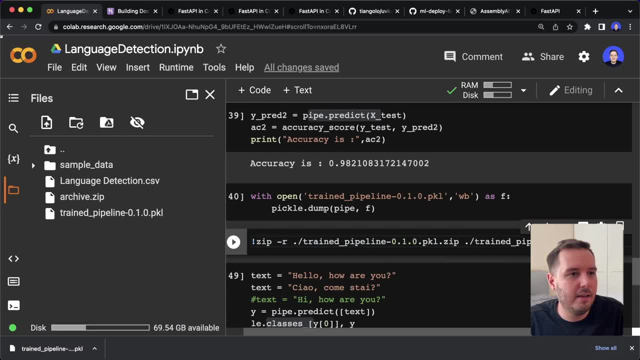 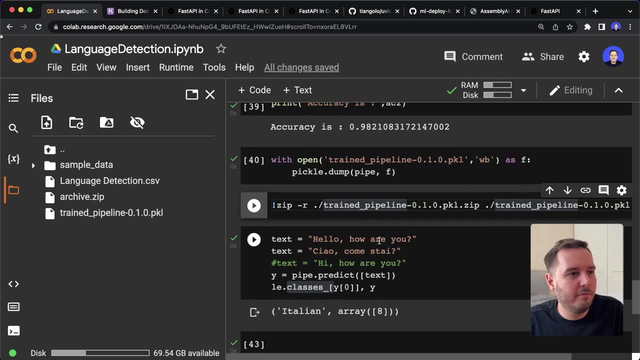 mark sip, and then you give it the name of the zip file and the name of the folder, And then you can download the zip file. So now we have this And finally, let's test this one more time. So here we have the text, And if we run this, then we: 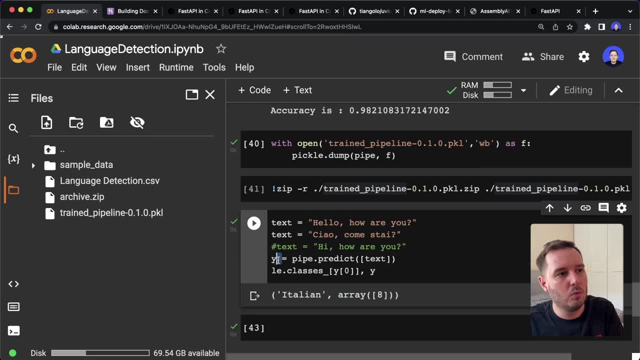 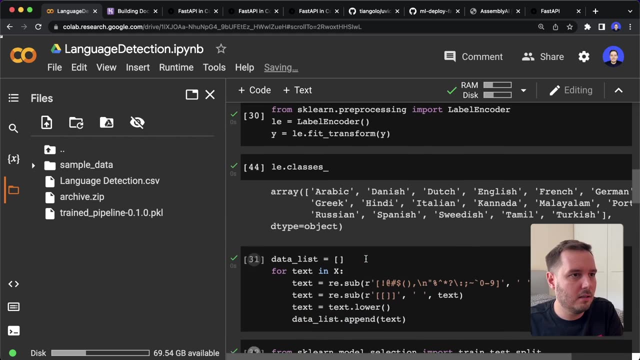 see this is Italian And we can also see that y is only this number eight here. So here we actually apply the label encoder classes to get the actual language, so Italian. So I printed this in the top. So here are the label encoder classes. So we also have to. 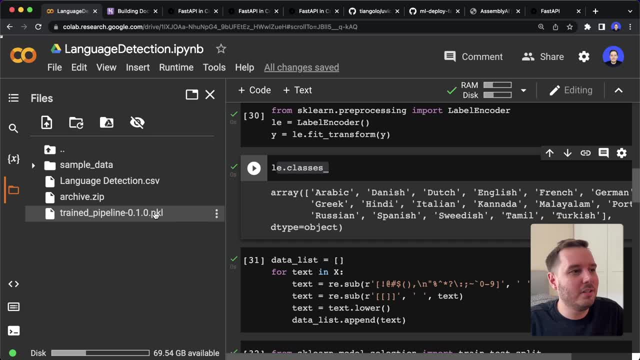 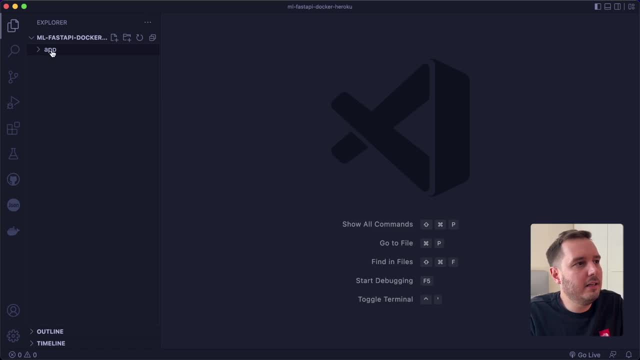 get this for our code And yeah, now we're done. So now we can use this model and build our app. Now let's create the fast API app And for this, in the root directory, let's create an inner directory app, And in here we will put all. 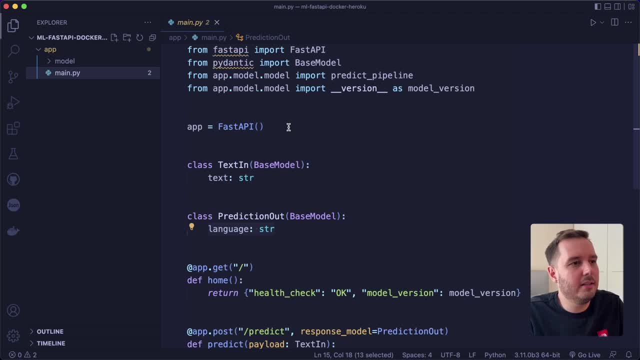 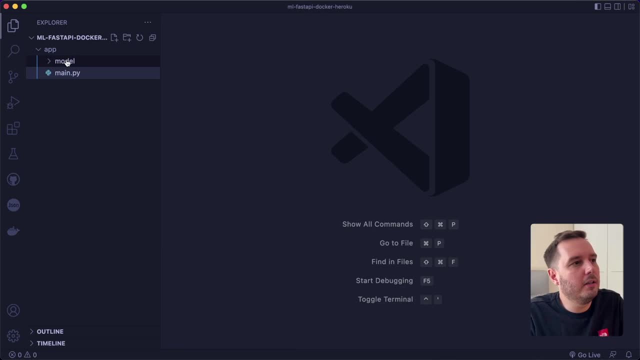 the code. So we have one main dot pi file. this is where we will put the fast API endpoints, And I go over this in a moment. And then we have a inner model directory, And here I start the downloaded pickle file, the trained model, and then another file that I called model. 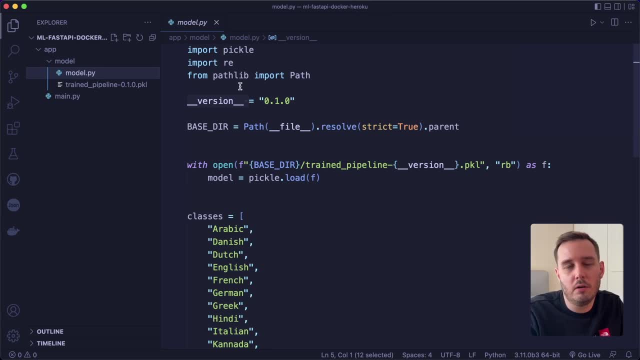 dot pi. So basically this is a helper file that does the model prediction. So here I hard coded the model version. Then I also use path and the path of the current file to get the base directory, And this is because the folder structure inside the Docker container can. 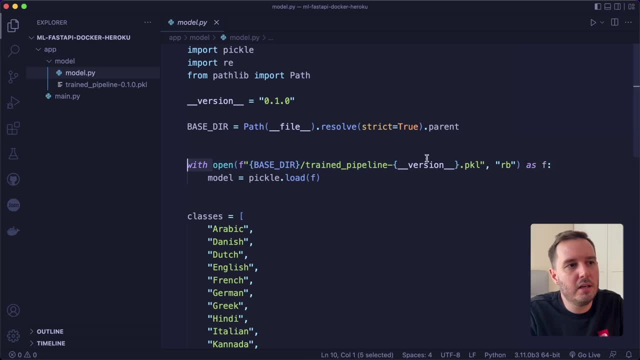 be a little bit different And I want to make sure that we can find this pickle file here. So then we can open this and make sure that this version corresponds to the file name, And then we can say: pickle load and loaded our model. Then here we have the classes. 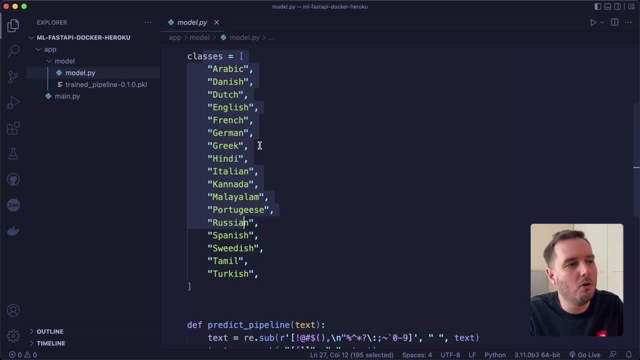 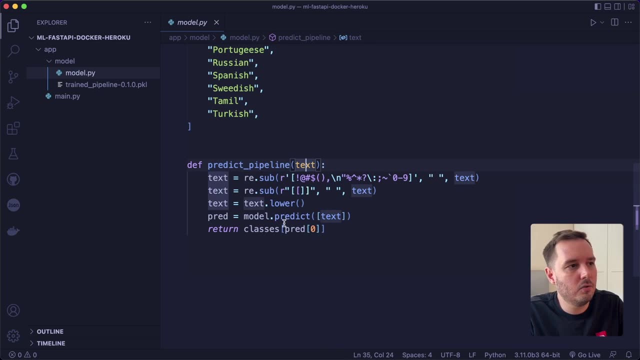 So this is from the label- encoder the classes in the same order, And then we only need one helper function, in this case predict pipeline. that gets the text. So this is a string, And then here we do all the same pre processing steps that we did in the notebook, And then 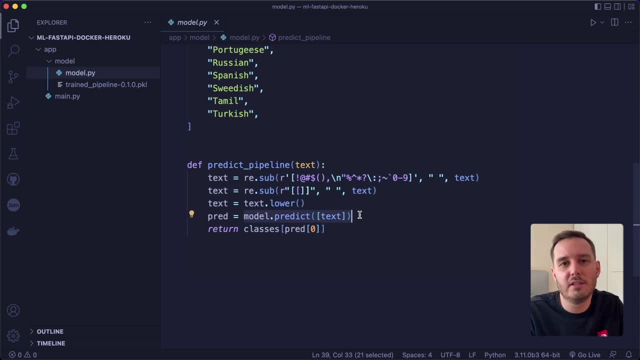 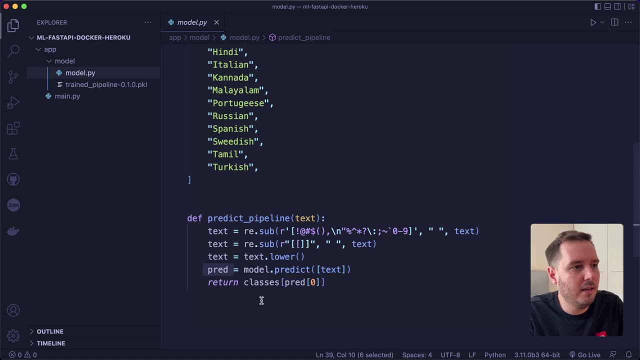 we can say model, predict we, because we now have only one step with the pipeline object. So then we get the prediction and this is a number. So then we have to access the index of the classes and then we can return the language. So this is the modelpy. And now 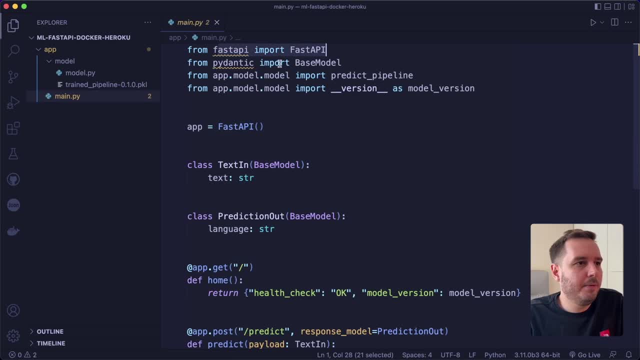 let's go to the mainpy. So here we import fast API and base model from pydentic. I show you what this is doing in a moment. Then we also import predict pipeline and the version as model version- and be careful to start your path with app. So appmodelmodel for this. 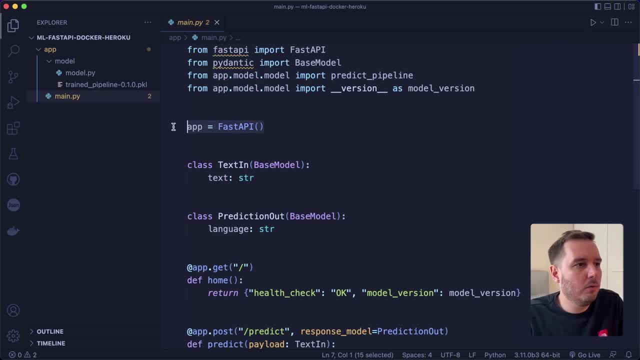 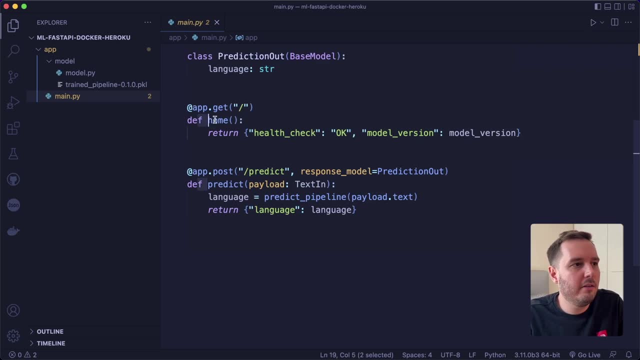 file And then it also finds it in the Docker container. Then we create the app and in fast API it's super simple to create your endpoint. So it's very similar to flask. we define a function and then decorate this with appget or apppost. So I often like to have a endpoint for a health check. So 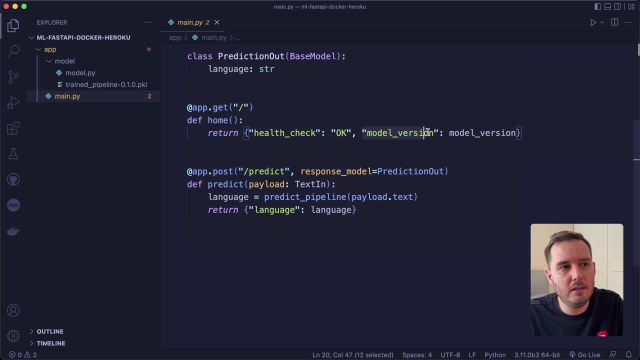 here we simply return health check, Okay, And here also the model version for additional information, For example. you can also return the API version here. And then we have one predict endpoint. This is a POST endpoint And in here we simply call predict pipeline and put in the text. 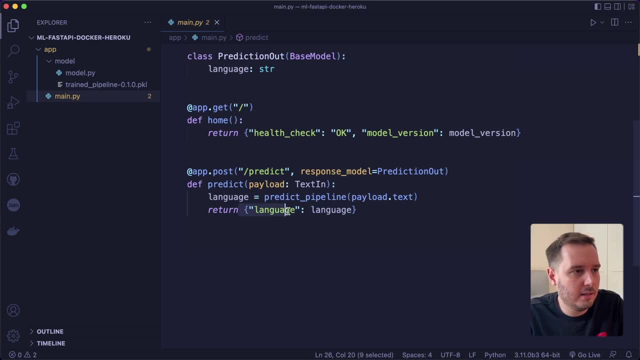 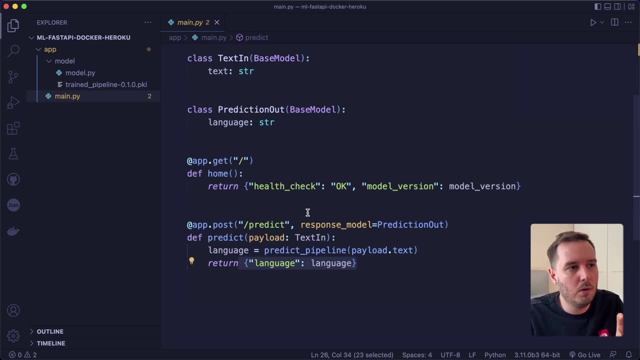 and then we return the language And this is a dictionary. And now to make sure that we pass the correct data types to this API when we send the data. So the input we want to have should be a string And fast API works with type hints, So for this we can define. 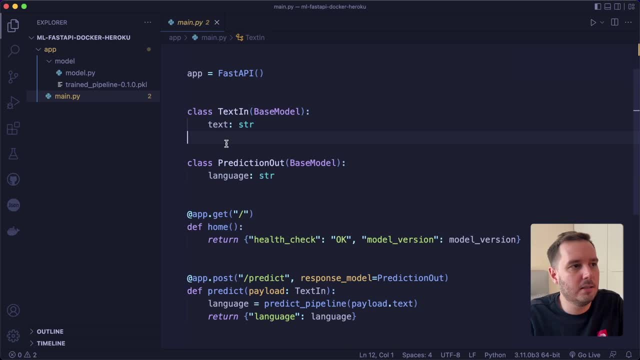 a class stand text in that inherits from base model And this should only have one field. this is a text, this should be a string. And now when we send the data and this is not a string, then fast API can detect this for us automatically and then raise an error or show an error in the API And this 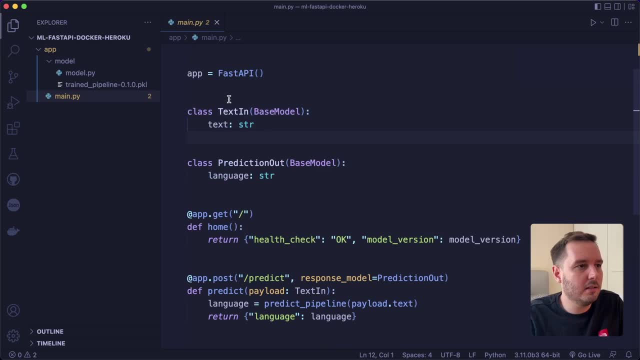 is super cool, a super cool feature of fast API. So this is why we use this base model, And in a similar way we do this for the output. So for the response we say prediction out, which inherits from base model, And here this should be one field language And this should also be a string. 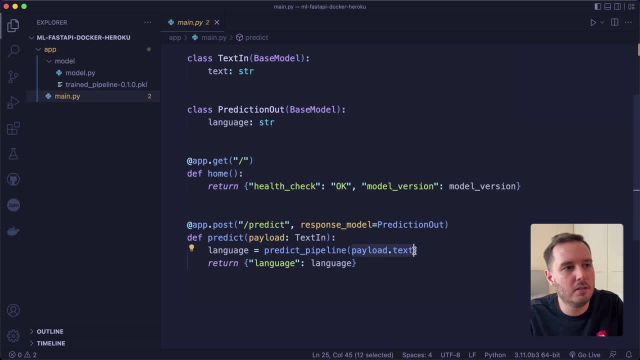 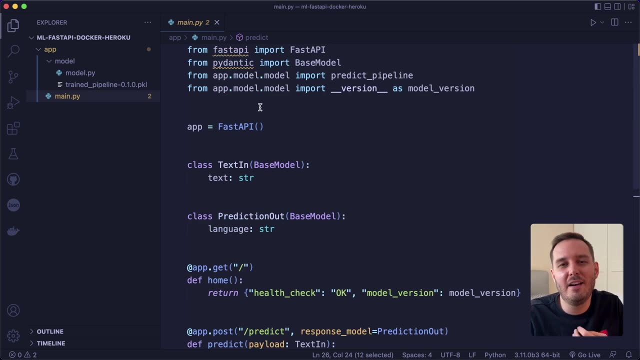 And then in the code here, we can access payload text, And we have to make sure that we have one field language, And this is basically all we need for this simple API, And now we can dockerize it. Now, to dockerize this, of course, you have to have Docker installed on your machine. 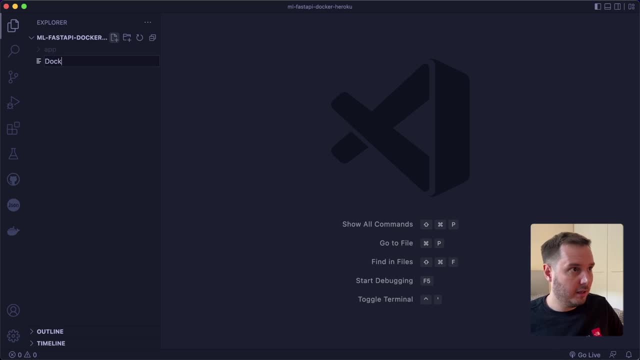 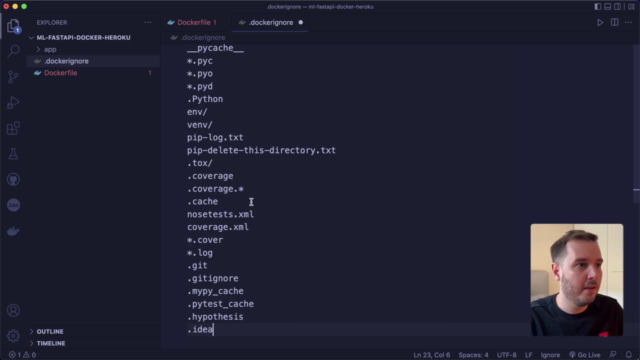 And then in the root docker directory we need to create a file that is called Docker file, And then it's also good practice to have a dot Docker ignore. this is similar to a dot git ignore. here I simply copy paste this from GitHub. you find this in the description, And this ignores certain files. 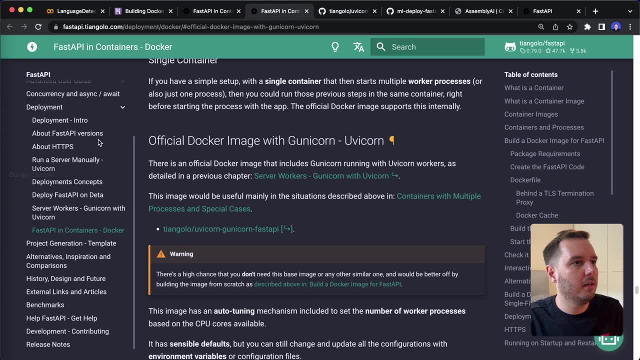 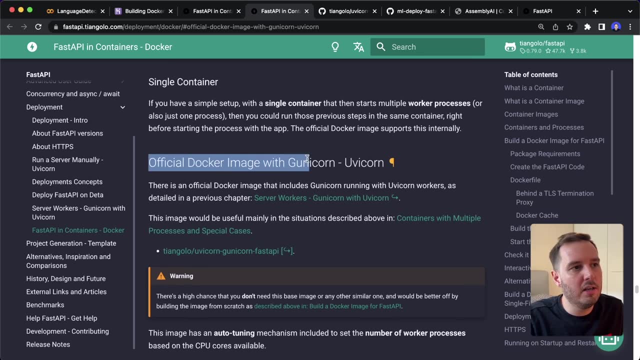 inside the container. And now for the Docker file, we can go to the official fast API docs. there's one section- fast API in containers, So I recommend reading through this because there are different ways of doing it. One way of doing it is to use the official Docker image with G. 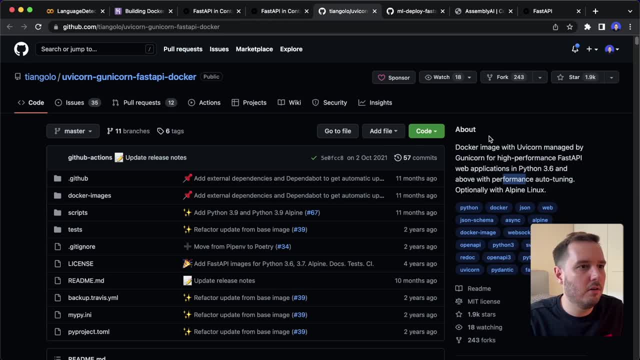 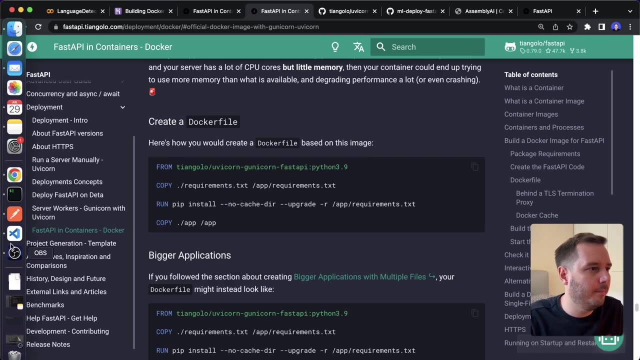 unicorn UV corn. you can also find this here on GitHub. So it says: Docker image with UV corn managed by G unicorn for high performance, fast API web apps And in order to use this, we can copy this code. So this goes in the Docker file And this is basically all we need to do And this uses. 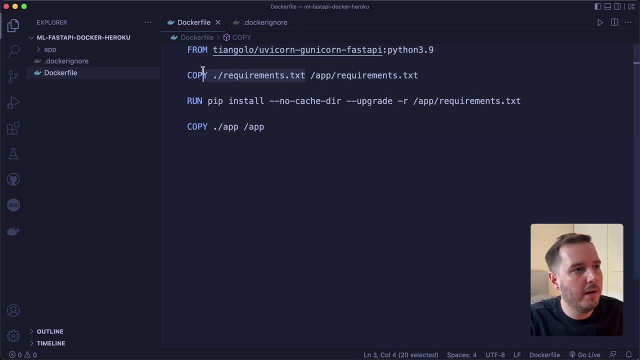 this base image, then it copies the requirements txt inside the container, then it runs pip install requirements And then it copies the app directory also in the container And that's why also we have to have this folder named app And then we need one file that is called require. 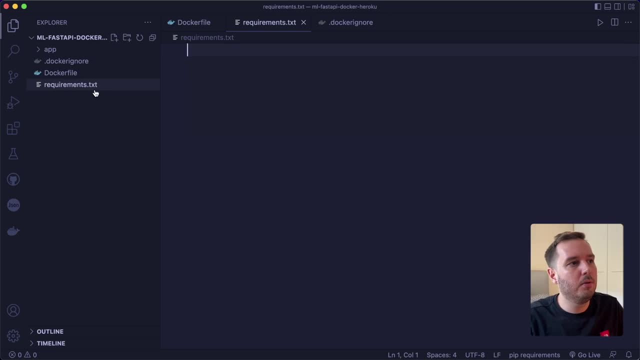 man's dot txt And here we put in all the dependencies. So in our case, since we already use the base image, it already includes fast API, UV corn and G unicorn. So the only missing dependency in our project is scikit learn. For example, if you use TensorFlow, then you. 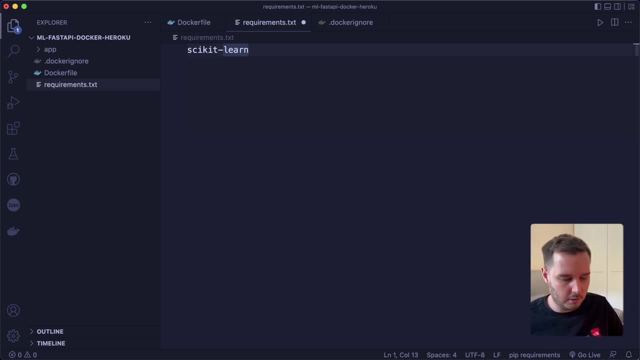 can put in TensorFlow here or pytorch And, for example. it's also important to mention, or worth mentioning, that you can use TensorFlow dash CPU oftentimes because you don't need the full version, and then your container will be much smaller. So 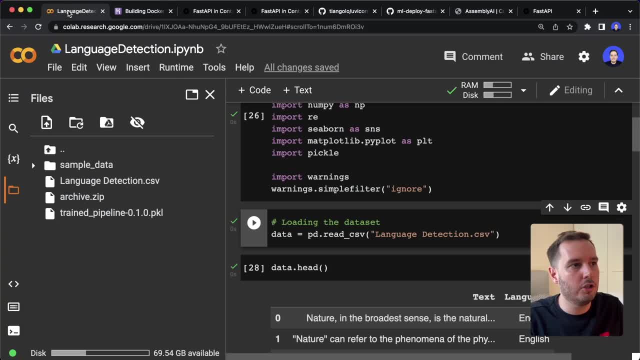 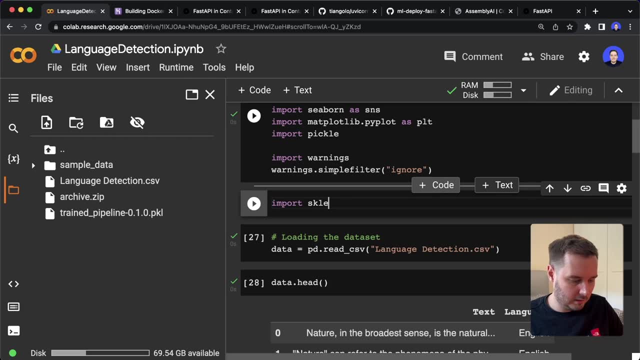 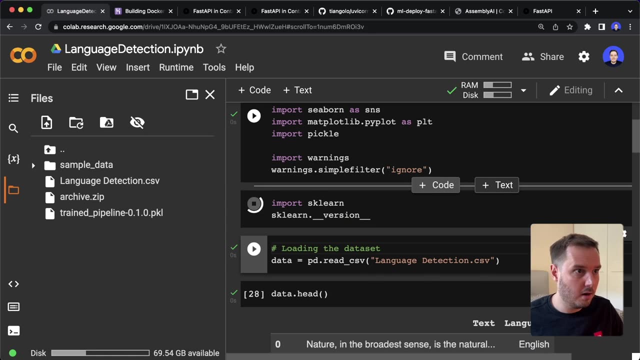 So then it's also good practice to pin the version. So for this we can go back to the notebook And then in here we can for example, say: import SK learn and then SK learn dot underscore version. this should give you the current version And then we can copy this. 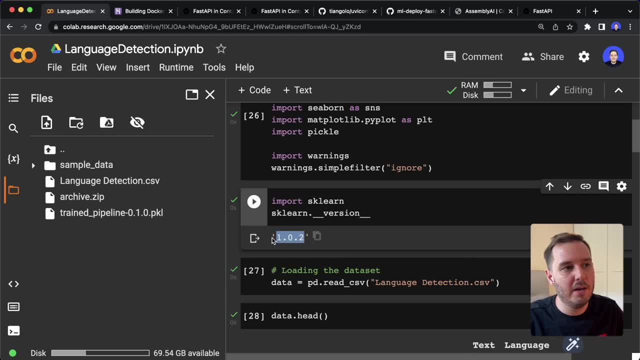 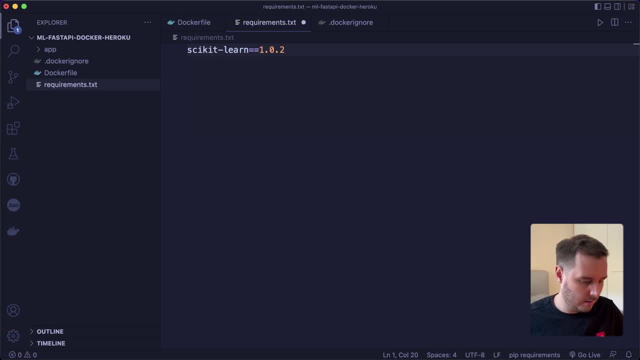 So it's 102.. So it follows the same pattern: major, minor patch. So let's go back and say: do this? let's say txt efficient is here. we need a property, sort of. I think we should send it a little bit faster. Let's just try it. 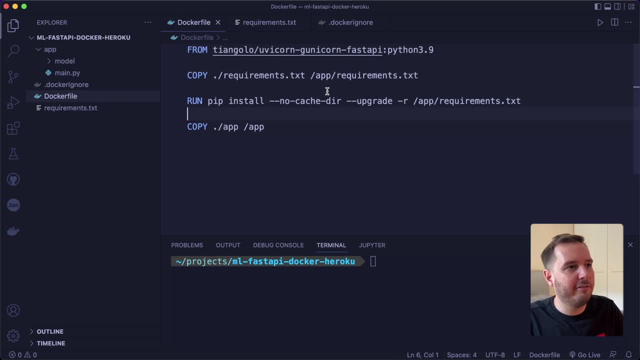 Cool, That's easy. So then, the rest of these fields we already referred to, in our case the about native MARThhab file we are talking about, without the traditional volume, ktl, which is basically acting as a dot project, We can now make a multi value. I mean a part. 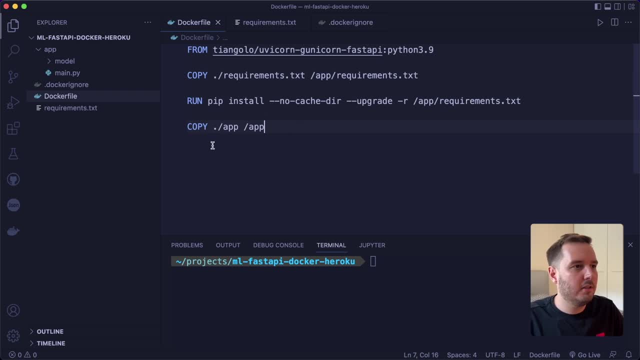 of one source or not just the way that we want to coordinate one difference between one order. As this comes through the definer, we can get any calls that we like, whether valid Patriot is an app, file, call, whatever else we need it to be In our case, just simply. 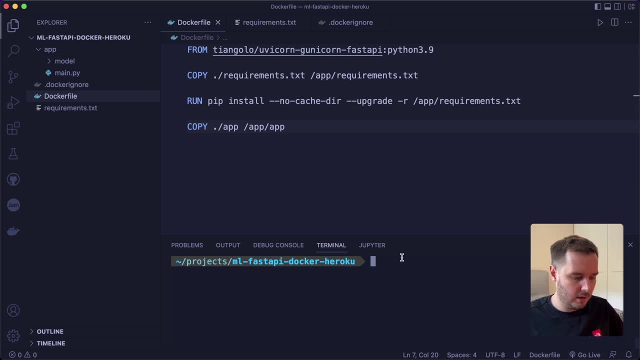 I characterizes the final value by putting it in the normal power file here instead of passing it through the app slash app. And now save this. and now we can say Docker builds and then minus T and give it a name. here I call this language detection app and then a dot for the current folder. 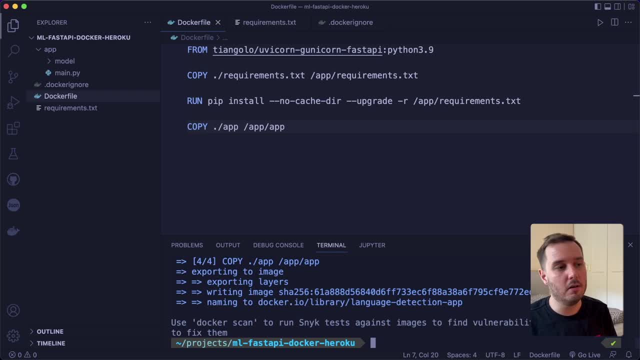 and then hit enter And now this will build the Docker image. And now this was already done. So if you do this for the first time, then this might take a few seconds or minutes. So now we have this and now we can run the container by saying Docker run, And then we. 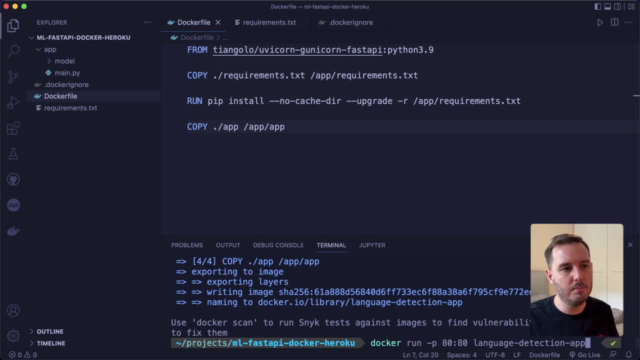 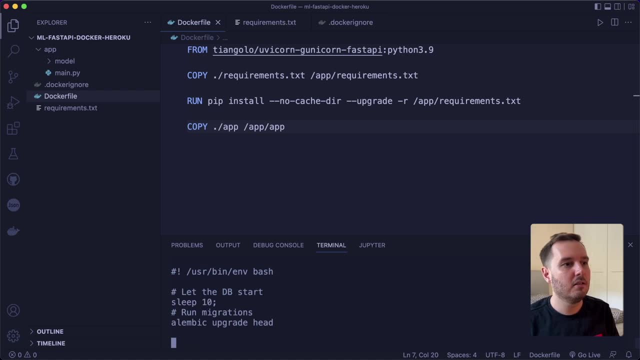 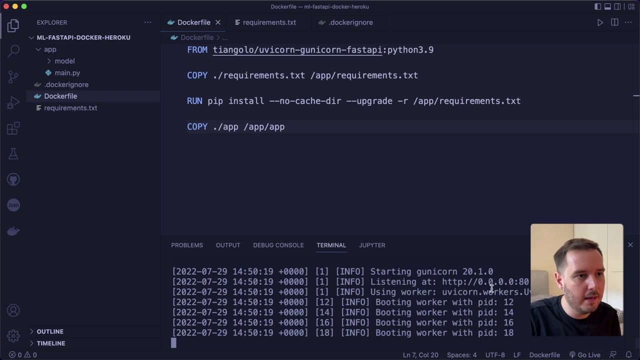 map the port from the Docker container to our machine by using 8080.. So this is port 80.. And then the name language detection app. So now this is running and starting, And now you should see that the UV corn workers are starting and it's listening to 000, port 80.. 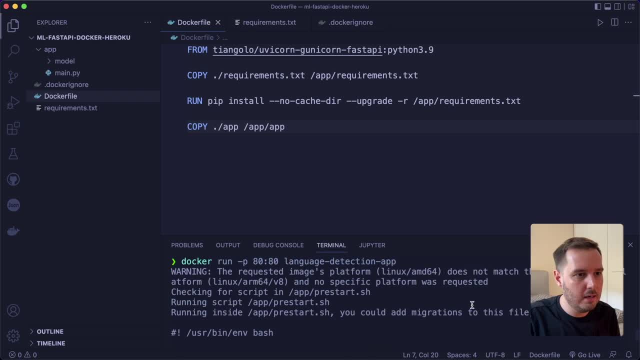 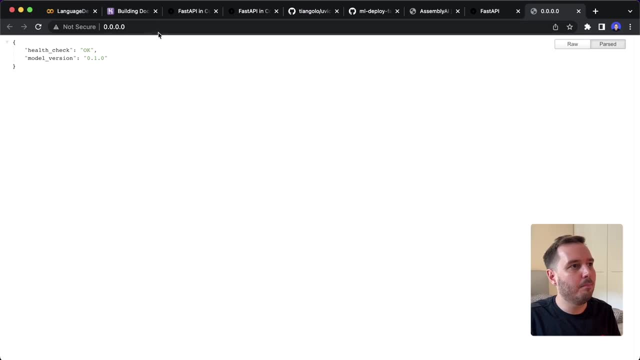 So basically, this is our localhost port 80.. So now we can find this and then go to the srout And for the base route, this is a get request. So this is working, health check okay and model version is 010.. So now we 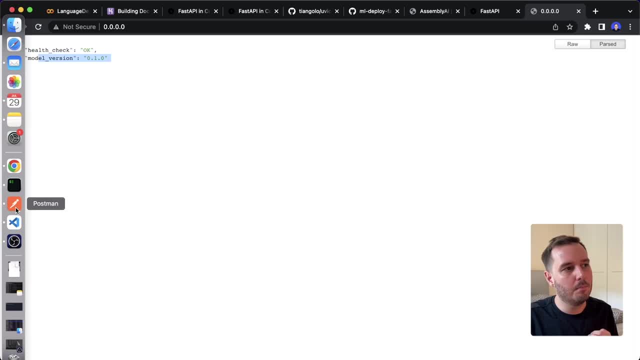 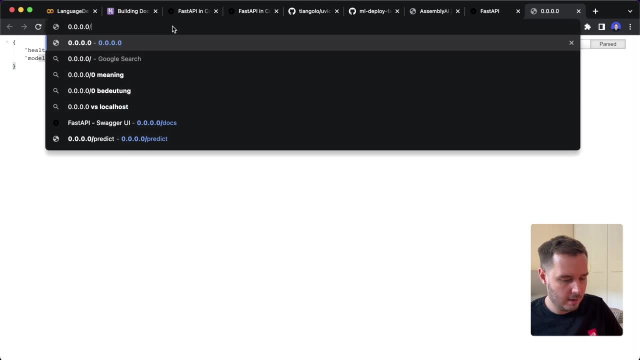 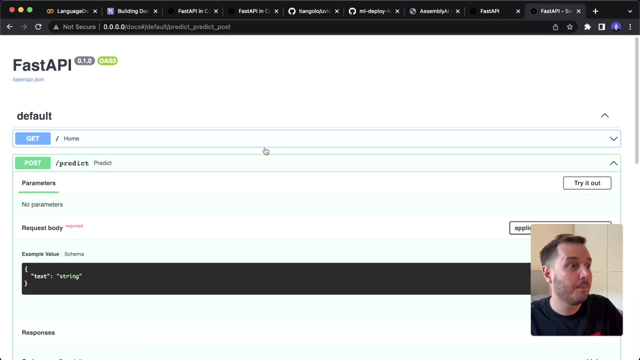 can, for example, use postman to send a post request. Or what's really cool with fast API is that we could automatic documentation by using slash Docs, And here we can see all the endpoints. So we have the home And we have slash predict, And then we also can try this out. And as you can see it, 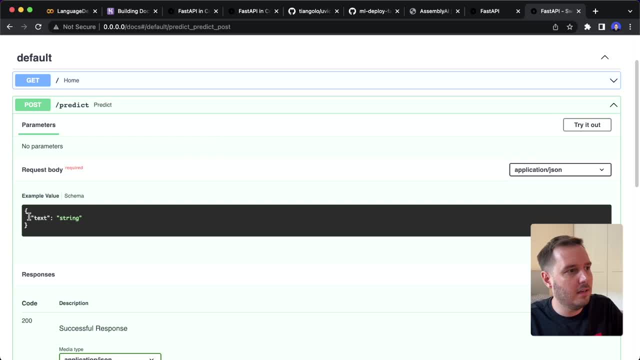 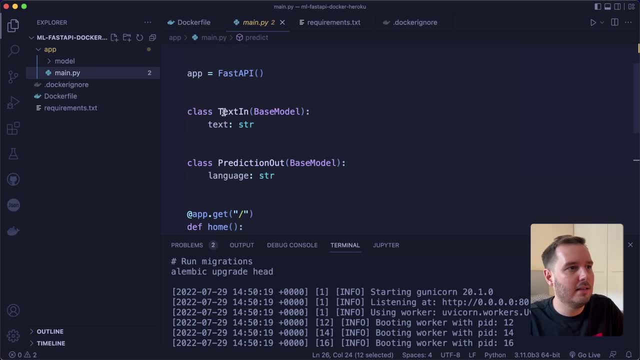 it knows that we need this schema with a text field and then the string. And this is because, if we go back here, we defined this as a base model with text, so the text and it needs to be a string. So that's why it knows that we need these fields And then we can click on try it out. 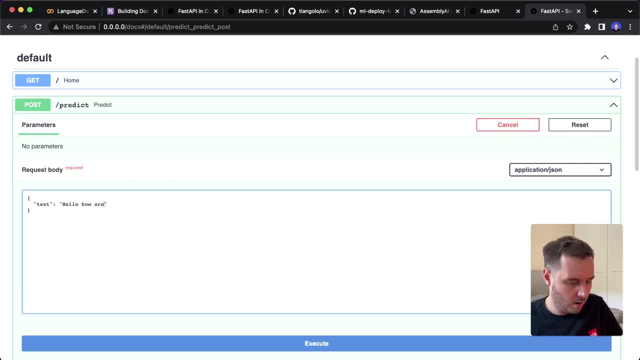 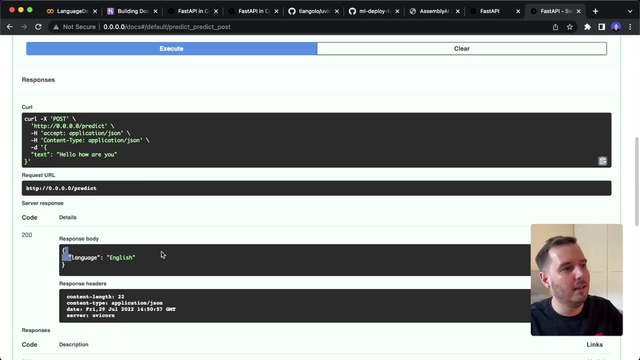 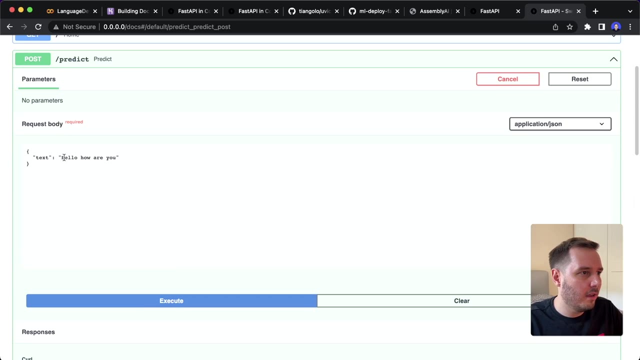 And let's say, Hello, how are you. and then execute, and then we get the response directly here and can see language English. You also get the curl command. if you want to try it from curl, So let's try it with a German sentence. So let's say, Hello, we. 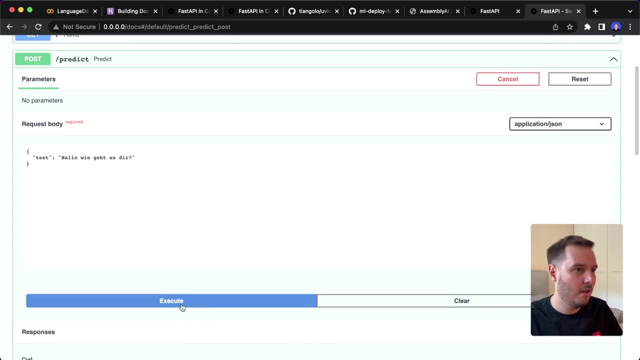 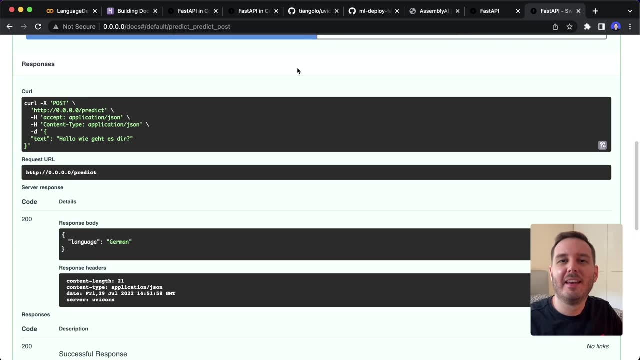 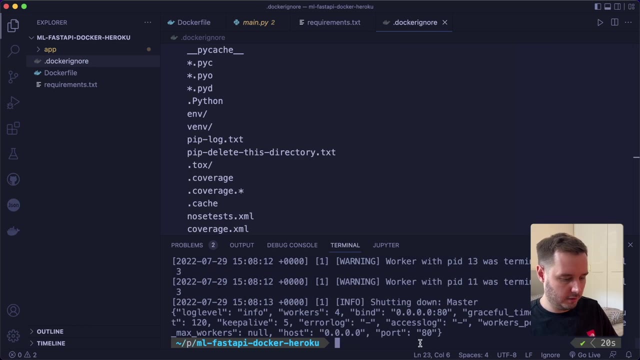 create a steer question mark and then execute this, and then language is German. So this is working. So now it's last step: let's deploy this to Heroku. And now we can deploy the container everywhere we want. In our case, we do it on Heroku, So let's actually stop our local container. 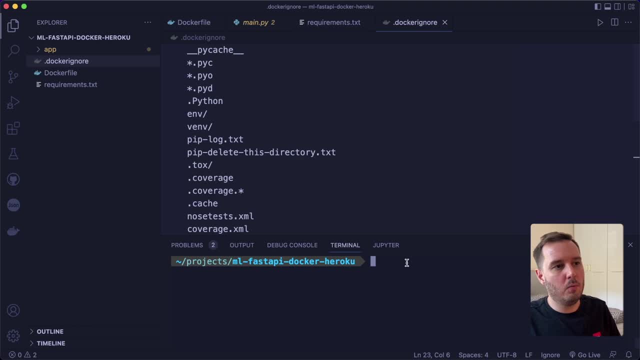 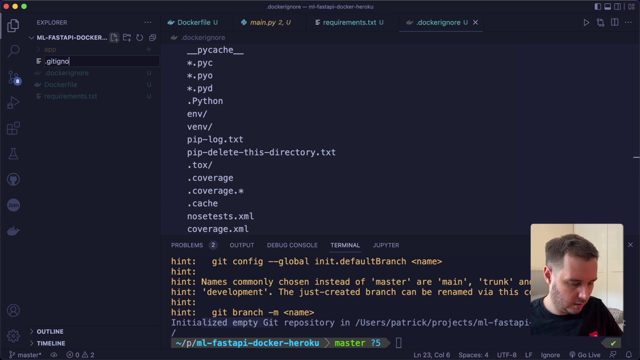 and clear this. And now, the first thing we want is a git repository. So we can say git init, And of course you have to have git installed on your machine. This will initialize an empty git repository. then I also want to add a dot: git ignore. So here we also ignore some. 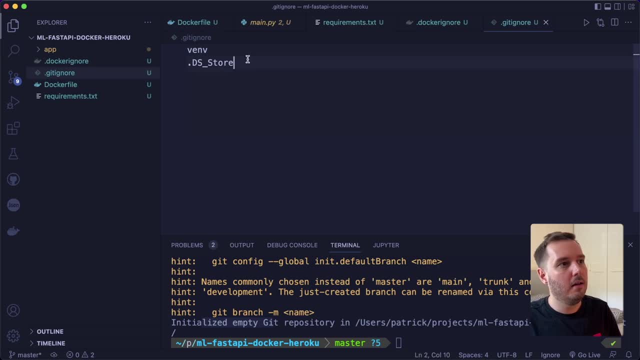 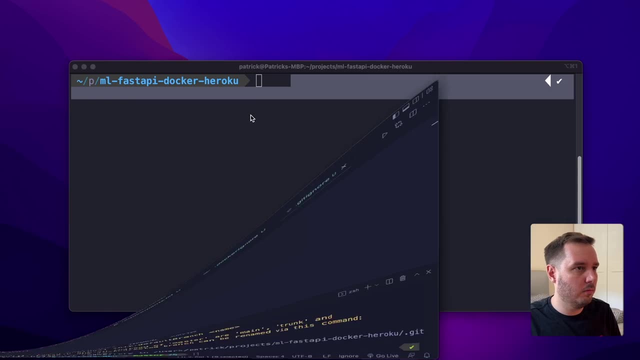 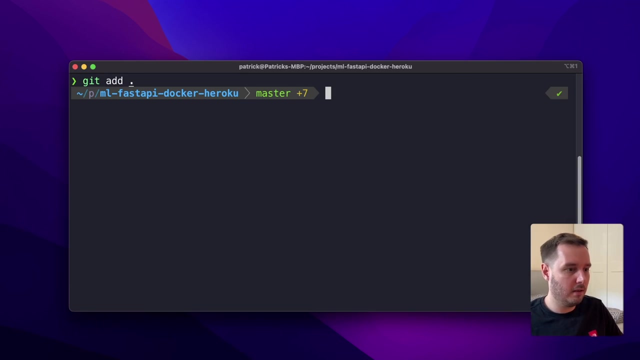 files and folders we don't need. So I only ignore the virtual environment and this file. And now you could continue in this terminal. I actually want to switch to my normal one. So here we now say: get at dots, so everything, So we can check it. status that, all these files. 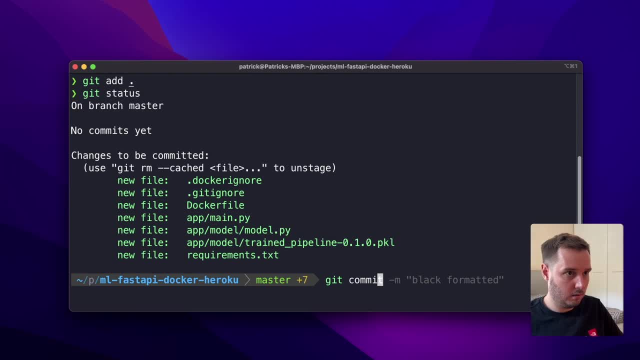 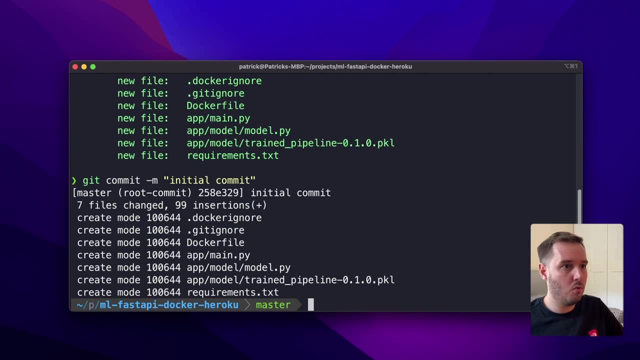 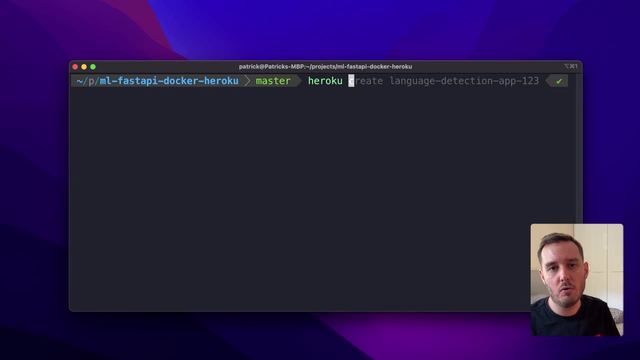 have been added And now we can say git commit and give it a message. So let's say initial commits And now we can start creating our Heroku project. So for this, of course, we need to have a Heroku account and the Heroku command line interface installed, And now we can do everything. 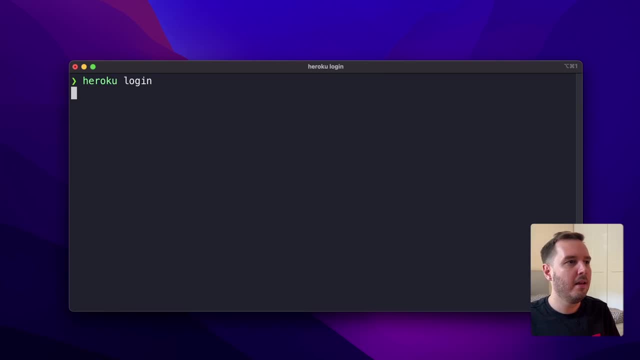 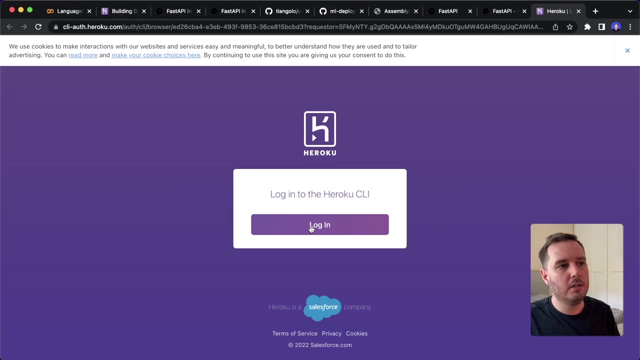 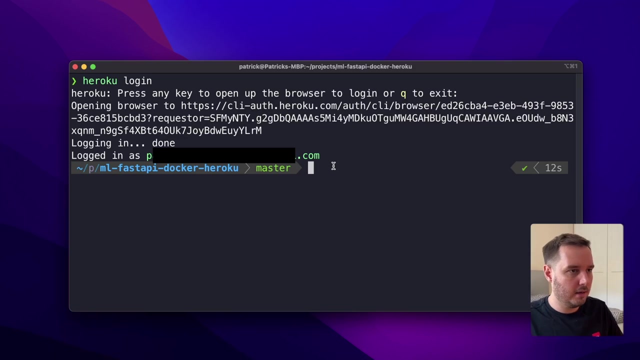 from the command line. So first we say Heroku, log in, And now this should open the browser, And then here you should be able to put in your credentials. So I think I already did this and this should be stored. So yeah, so now we can go back and see we are now locked in And 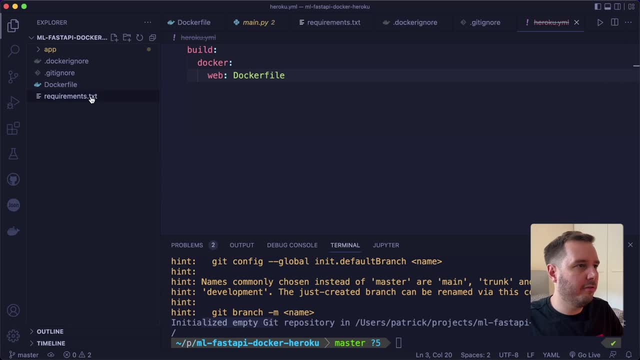 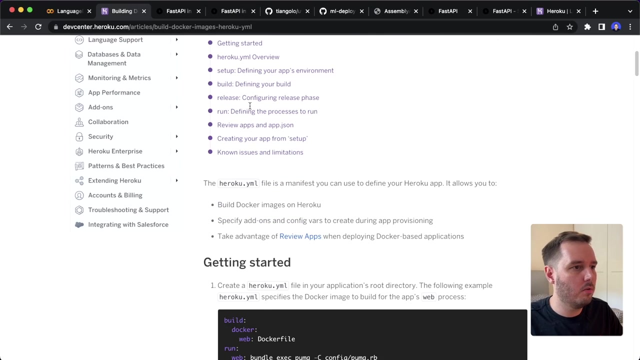 now, before we can continue, we actually need one more file, also in the root directory, And this is called Heroku dot YAML, And for this I can recommend a documentation site on the official Heroku dev center. building Docker images with Heroku YAML. 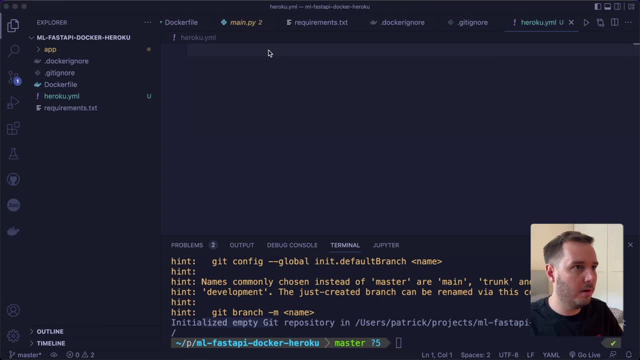 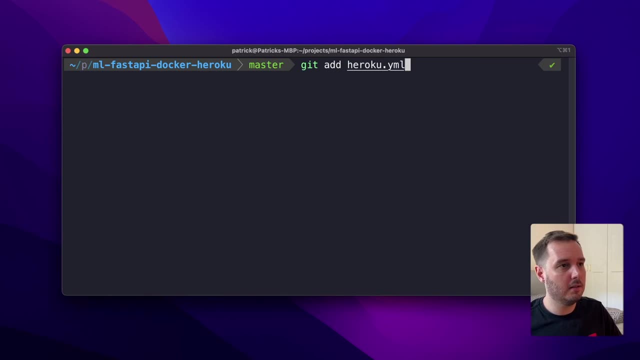 So basically we only need this part, So let's copy and paste this in here. then of course we have to add this to get again. So we say, get at Heroku YAML. And then we say get commit and add Heroku YAML as message, And now we can create a new Heroku project. So we say: 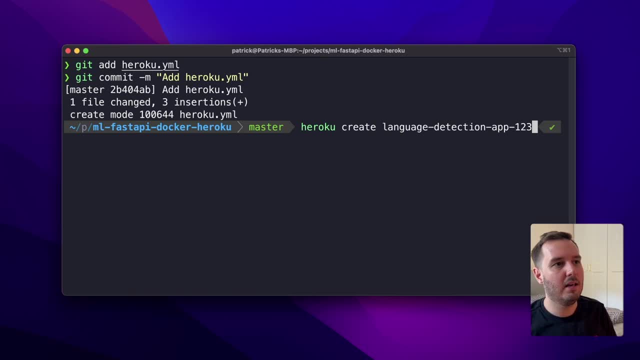 Heroku create, and then we have to give it a name. So let's use language detection app, And then it needs to have a unique name that is available. So let's try one, two and see if this works. Alright, so, this works. So now this will be the URL that we can use to access our API.